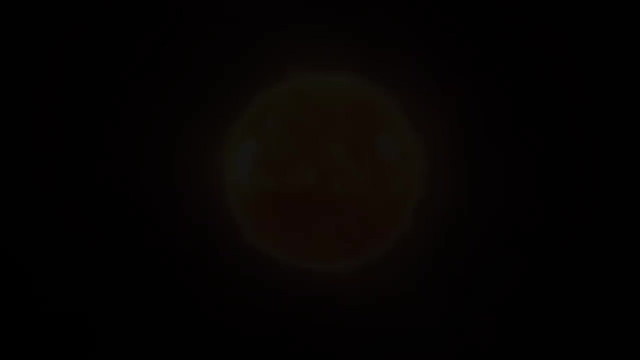 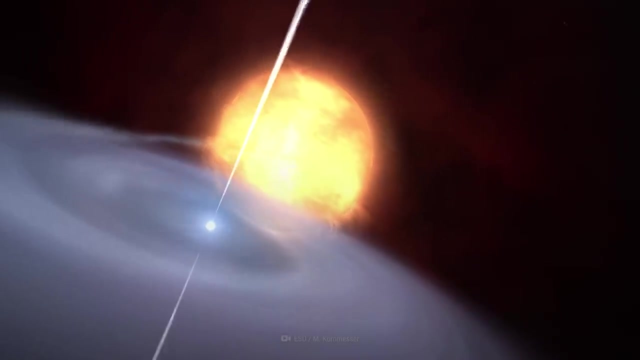 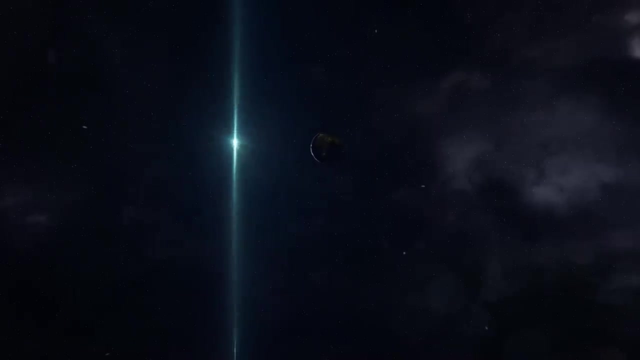 This is the Sun And this is a neutron star, But don't let its size fool you. Neutron stars are massive gravitational monsters And orbiting one wouldn't end up well for our planet. But what if we took just a spoonful of it? 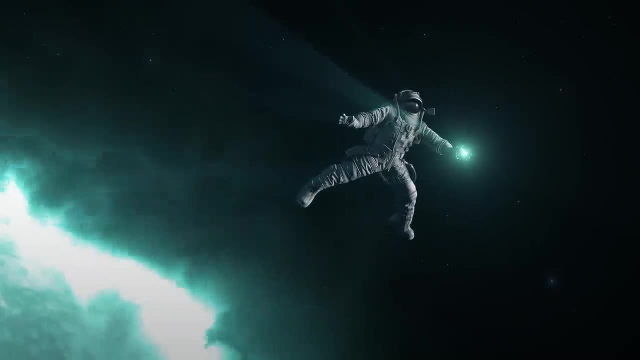 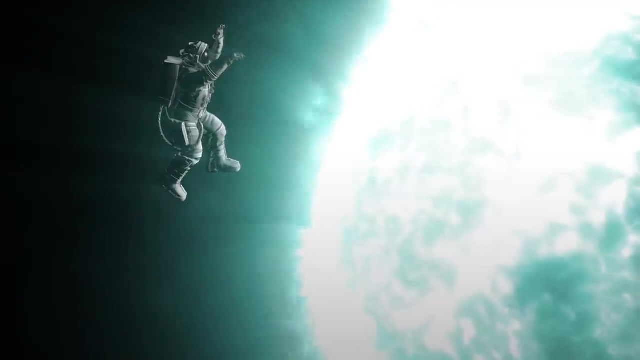 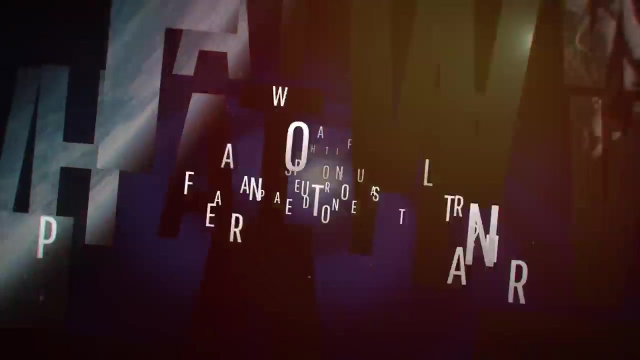 and transported it to Earth. Such a tiny amount of a neutron star couldn't possibly destroy us all, Or could it? This is WHAT IF, And here's what would happen if a spoonful of neutron star appeared on Earth, When a star about four times the size of our Sun. 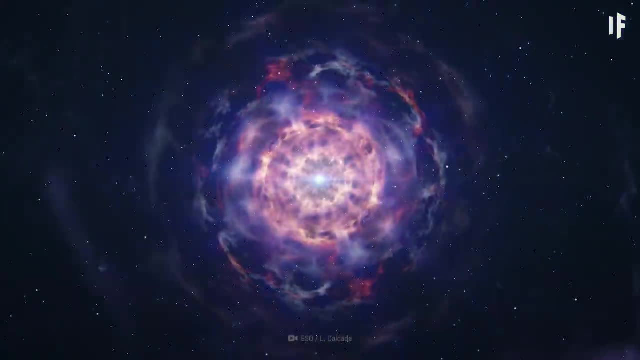 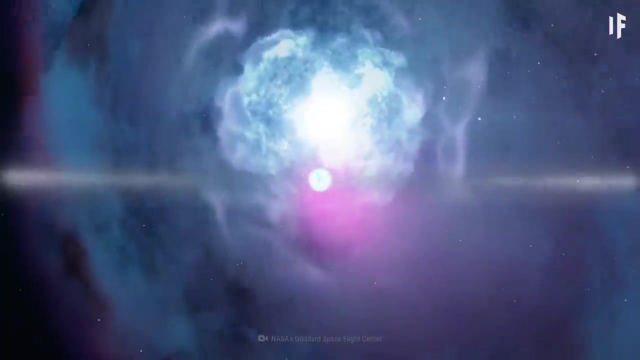 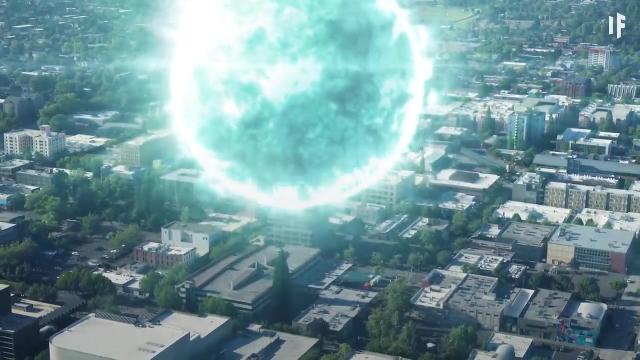 explodes in a supernova, it propels its outer layers into space, leaving only a dense collapsing core behind A neutron star. Neutron stars are very, very dense. They could have the diameter of a small city, but their mass would be 1.4 times the mass of our Sun. 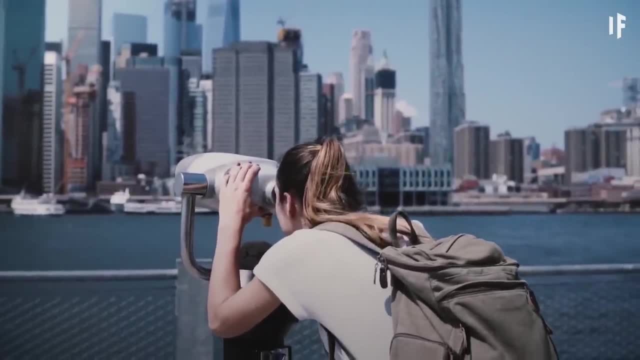 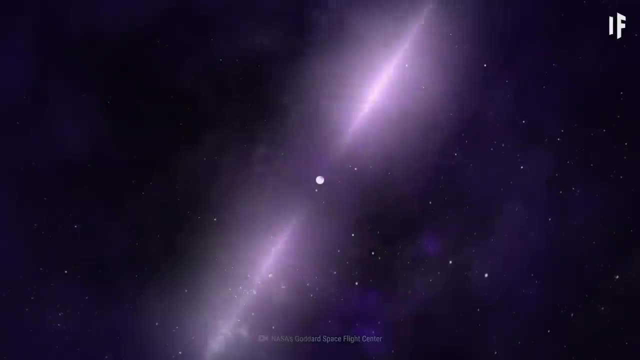 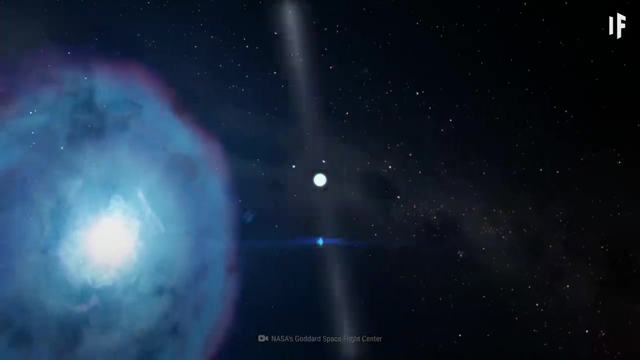 Of course, no neutron star will ever appear on our planet by itself. First, you'll have to grab a spoonful of it and bring it back to Earth. You'll find the nearest neutron star, nicknamed Calvera, 617 light-years away from Earth. 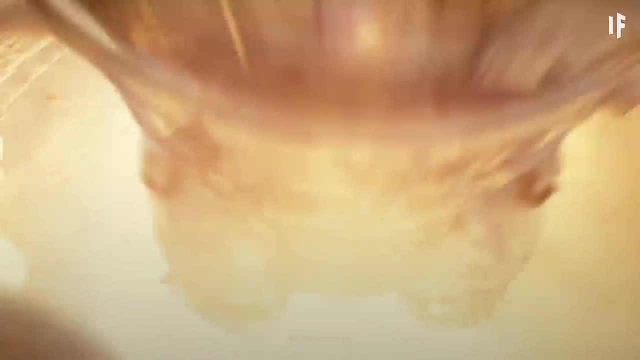 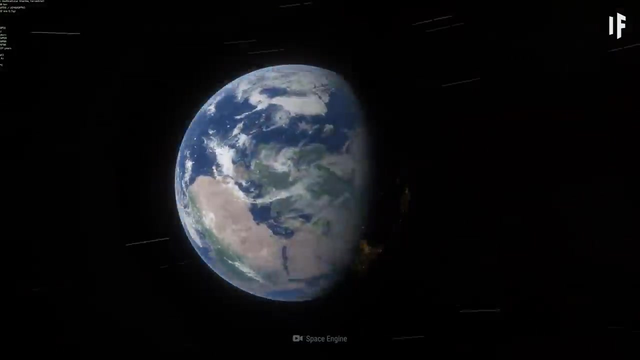 If you jumped in the fastest spaceship we've ever built, it would still take you 11 million years to travel to Calvera. I'll have to fast-forward here and meet you in the neutron star's neighborhood. You'd be trying to get your spacecraft. 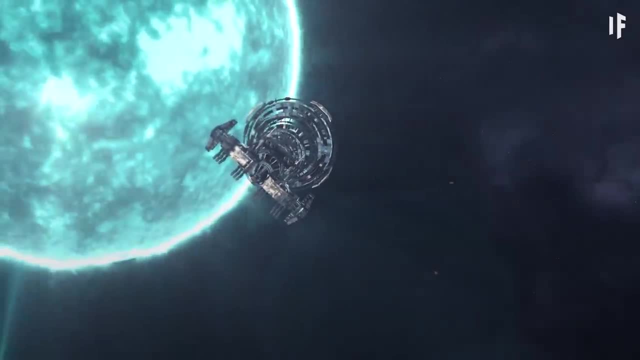 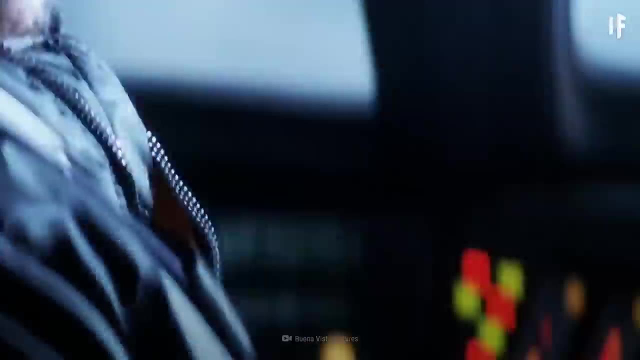 through a magnetic field that's tens of millions of times stronger than Earth's. Your ship's computers would be useless if they had any ferromagnetic materials like iron, nickel or cobalt in them. You wouldn't want any of those materials anywhere in your craft. 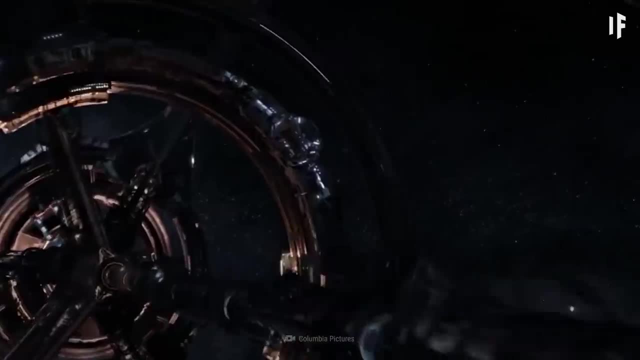 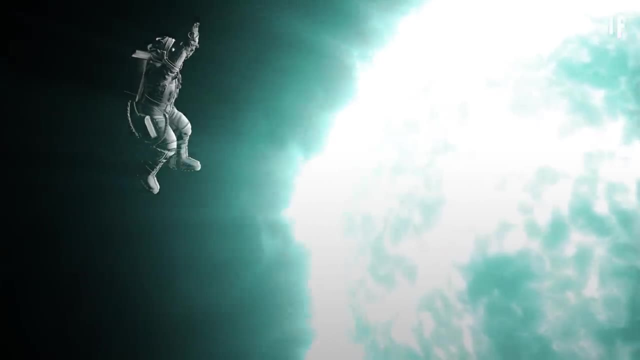 You'd have to dodge the electromagnetic radiation beams shooting from the star faster than you can blink. And then, when you finally managed to get to the surface of Calvera, you'd be immediately vaporized due to the temperatures being around 1 million degrees.